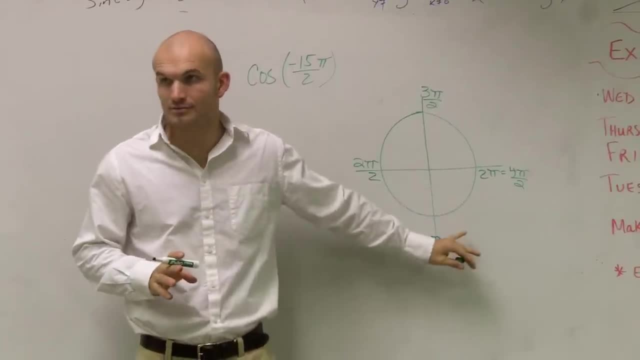 Yes, But let's say you didn't have a unit circle, right? Let's say you don't have a unit circle and you don't want to write one up. What we can do is we can rewrite this in terms of pi. 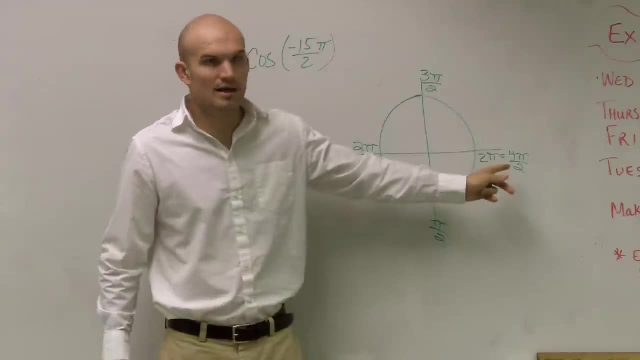 Because what they say is: when we just go around the circle, I'm just back to where I started, right, I'm just doing extra work, It's redundant, We don't need to. If I go around the circle, it doesn't matter. 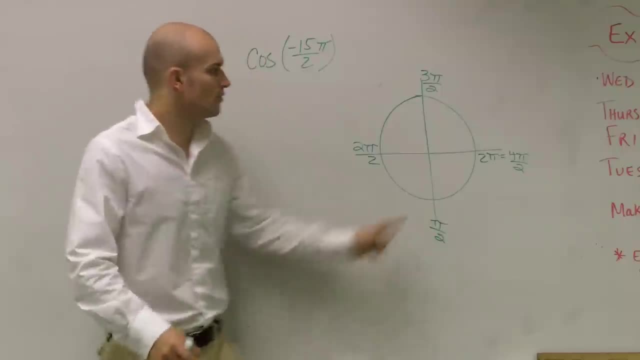 We just want to know where am I going to end up, right? So what is going around the circle all the way is what we call 4 pi over 2.. So what I'm going to do is I'm going to say cosine. 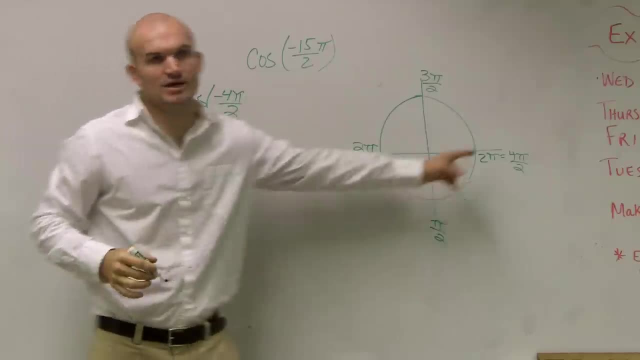 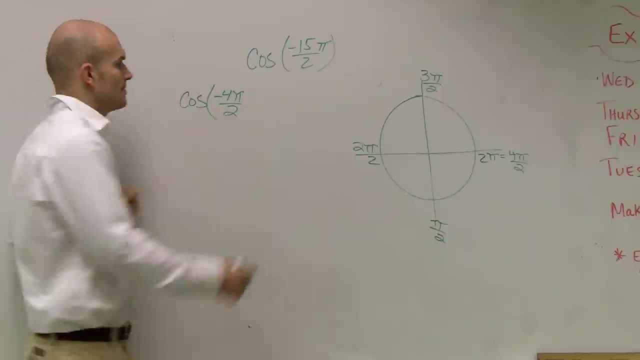 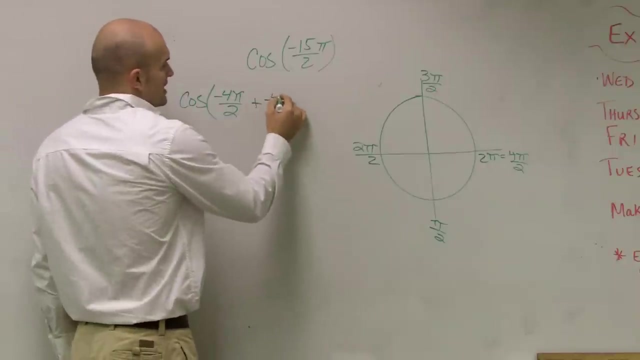 and I'm going to write it as a negative because we're going in the negative direction. okay, So this is going around the circle how many times? Once right, And then we can say, plus, We can go around again. These two added up. 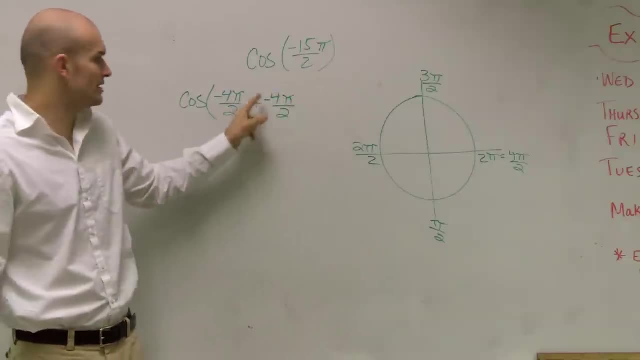 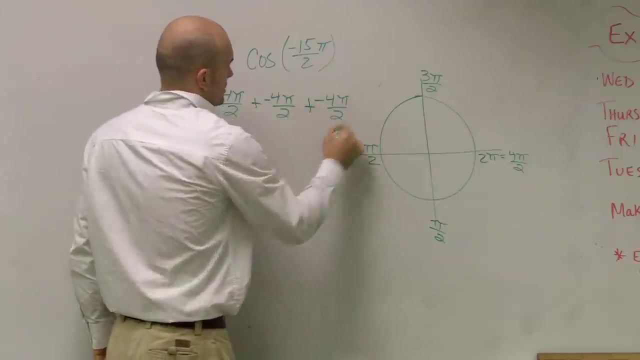 Does it get me to 15 yet? No, but again, what am I doing? Went around the circle once. Went around the circle twice right, Plus Now I go around the circle three times right. Have I still got to where 15 is? 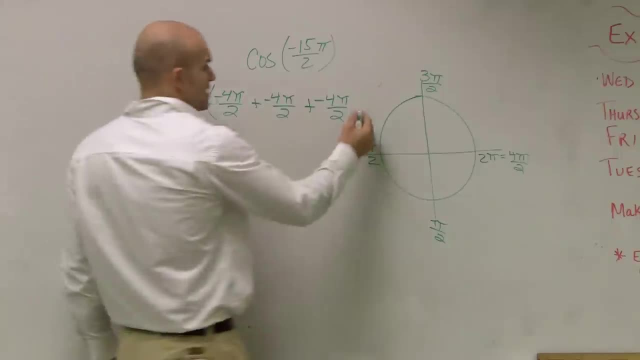 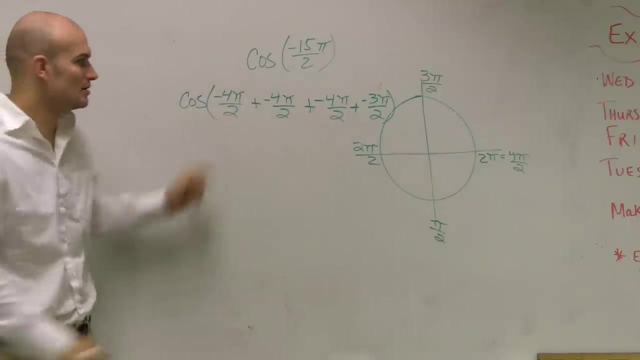 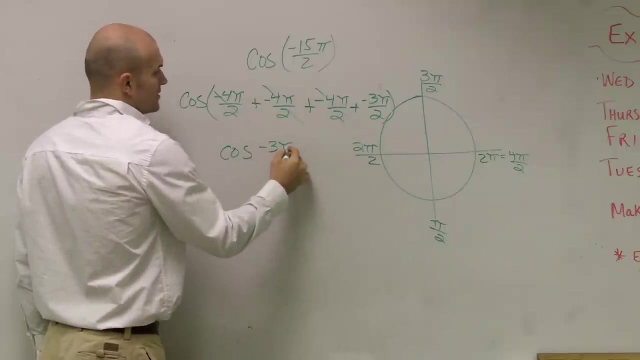 No, but what's going to be my remainder? Three Negative 3 pi over 2.. Now, since all of these are just going around the circle, we just need to evaluate. We don't really care about these, We just really care about cosine of negative 3 pi over 2.. 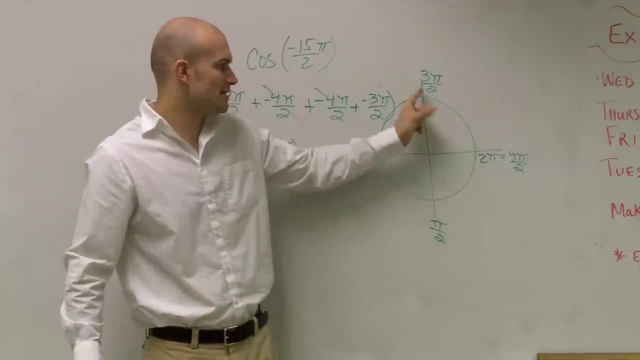 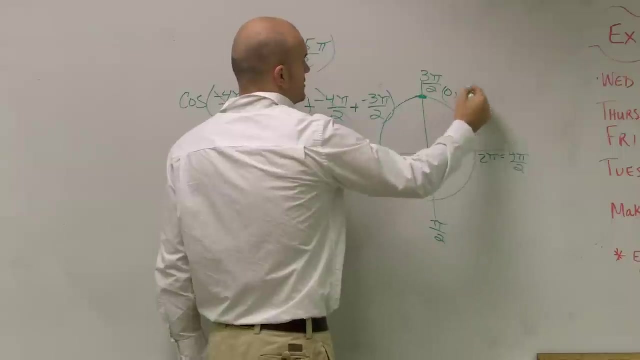 So what's the cosine of negative 3 pi over 2?? Well, here's 3 pi over 2 in the negative direction. So remember, this point is 0, comma 1.. The cosine is going to be 0.. All right, 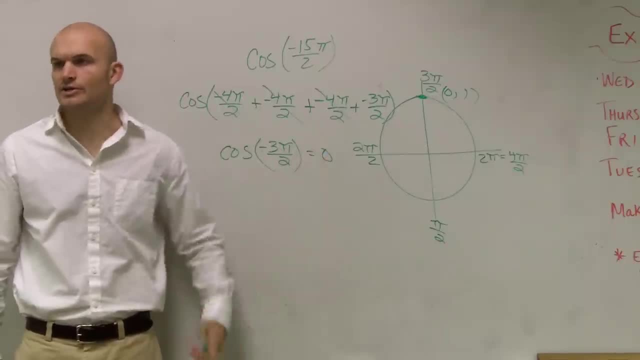 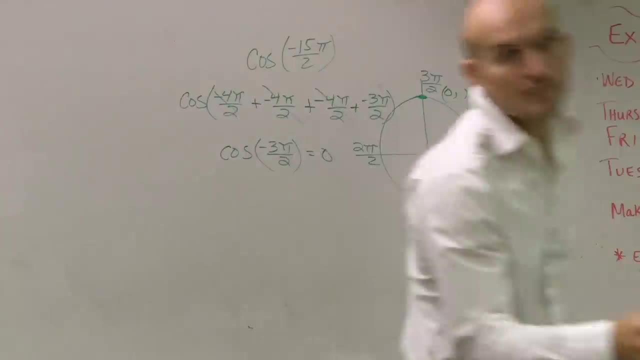 So, like I said guys, once you do enough of those, you can probably start calculating that in your head without having to draw the circle out. Yes, It's 0, because cosine is x, Exactly. So whatever our remainder is is our. 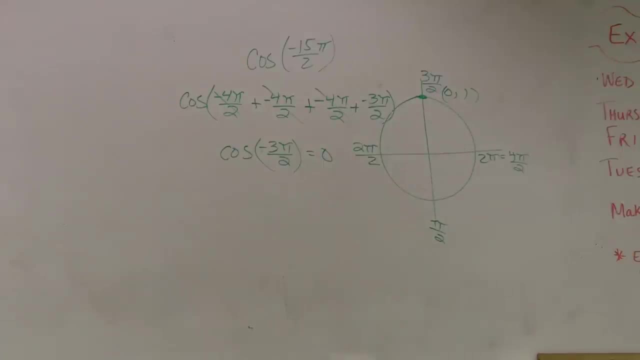 Yes, yes, You can think of it like your remainder after that. Thank you. 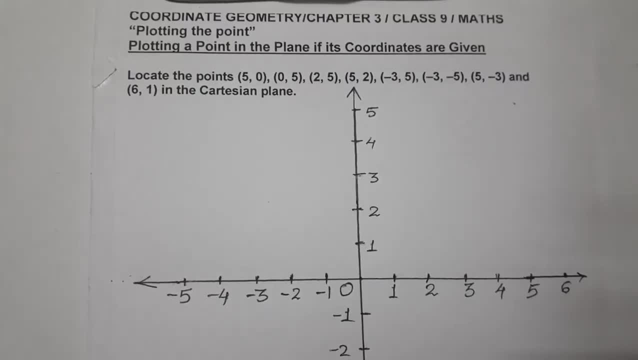 Hello students, today we are going to learn how to plot the points in a plane if its coordinates are given to us. So let's start. So see, some points are given here and we have to locate the points in this Cartesian plane.